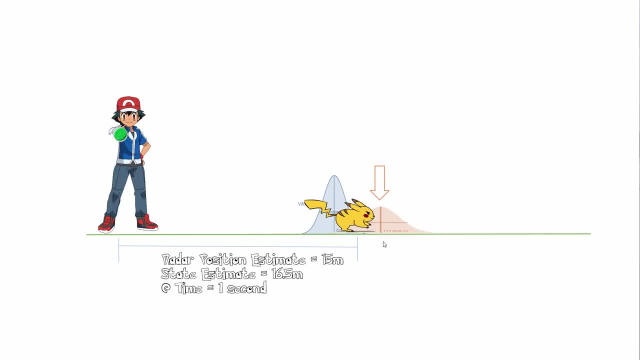 Do we throw a ball at around 15 meters Or do you throw it at around 16.5 meters? Now, it makes a huge difference, because if you throw your Pokeball a few centimeters ahead or behind, you know you're going to miss the Pikachu and it's going to run away. 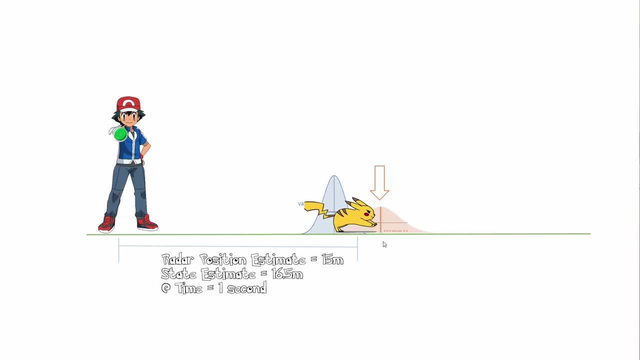 So we have to get this right the first time. We have to find the optimal estimate of where the Pikachu may be. So what do we use? Now for those who say: why don't we just use the average of the two? So we say 16.5 plus 15 meters. 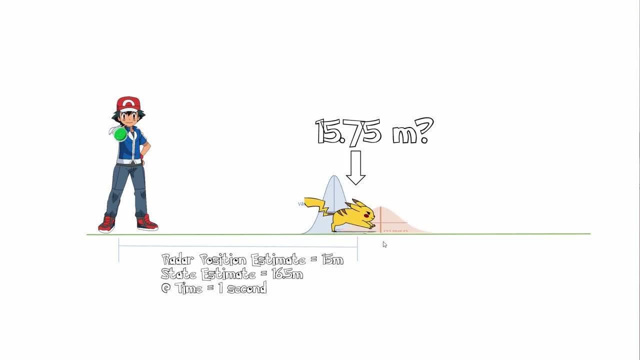 So we start by two and we get a halfway mark of 15.75.. But how do we know that the Pikachu isn't at 15.3 or 16.25? We don't know, And here we need accuracy, So we can't do that. 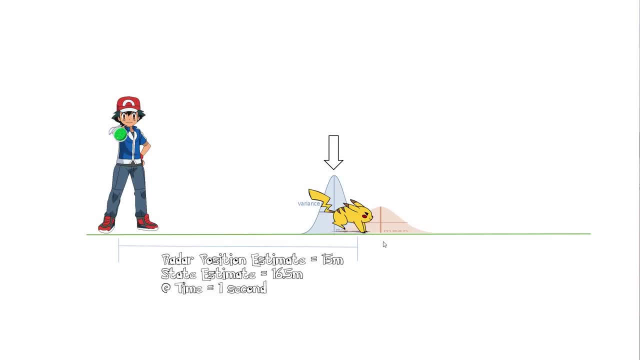 So a rather better way is to take the mean and variance of the Dragon Raider estimate along with the mean and variance of our state estimate And we combine it into an optimal estimate which will give us the best estimate of where the Pikachu will be. 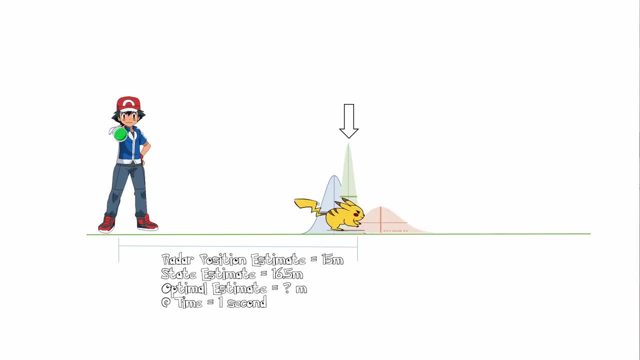 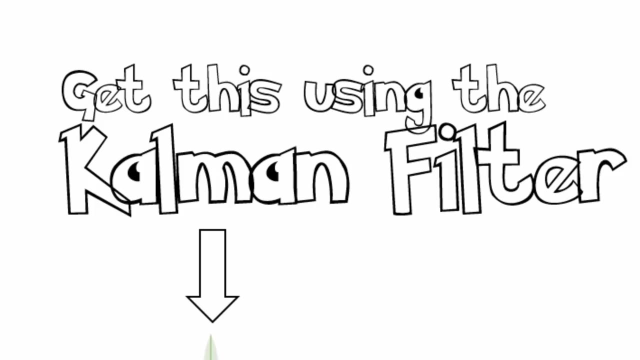 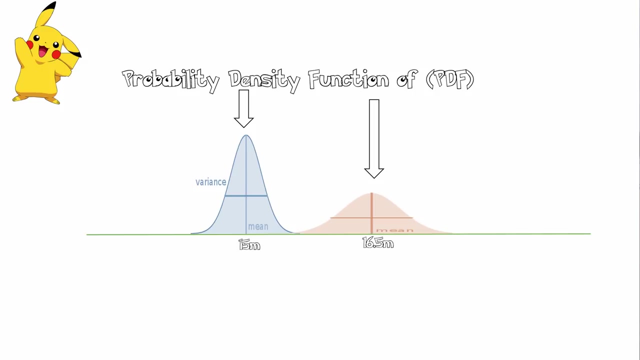 And that can be anywhere in between the two means. So how do we get this estimate? Well, I'm glad you asked because we can use the almighty Kalman filter in the background. So before we move on to what and how and what of the Kalman filter, 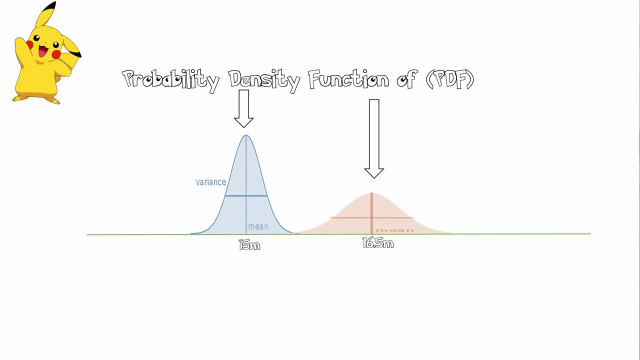 let's take a step back and look at the probability density function, or PDF, not to be confused with Adobe PDF. So probability density function is basically: we have highest probability, We have the lowest probability of one and then the lowest probability of zero And, as you can see, our measurement has a higher probability than our state estimate. 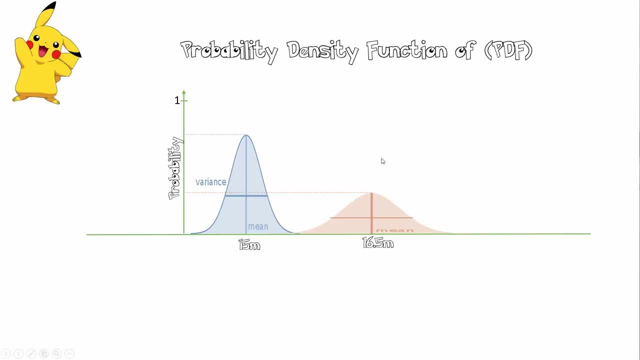 So we trust our measurements more, But there are also cases where our state estimate is much more accurate. And also, if there's misdetections in our measurement Now at the moment, why this is not so accurate, or we assume it's not accurate because the Pikachu may be running a bit slower, a bit faster. 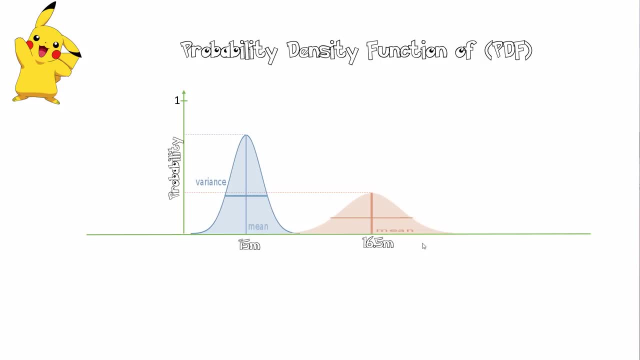 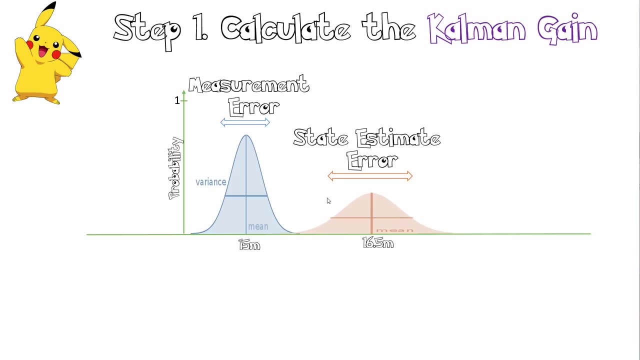 There may be turbulence along the way, It may slip on a rock. So we have to do a little bit more testing again. So we assign this a low probability for now. So step one is to first to calculate the Kalman gain. So we take our measurement error. 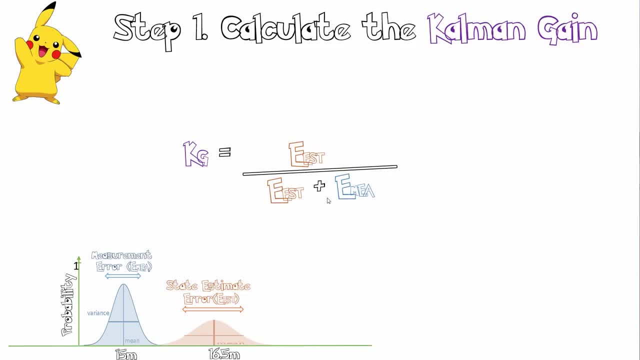 We take our state estimate error and we come up with this equation. So what this equation means is that we've got our Kalman gain, which is a combination of our error of the estimate, And over here we add our, the error of our measurement. 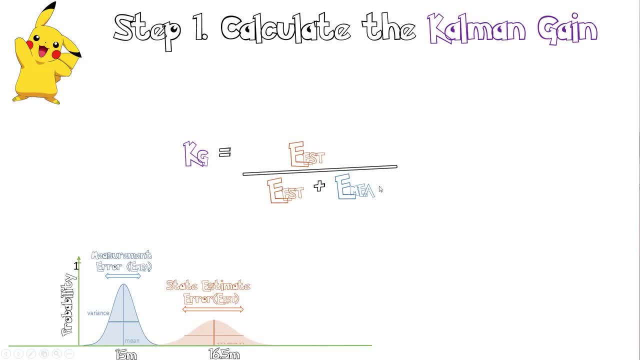 So what happens? if our error in the measurement is zero, Then this divided by this equals one. We've got a Kalman gain of one. If this is very, very low, If this is very large, we've got a large error. 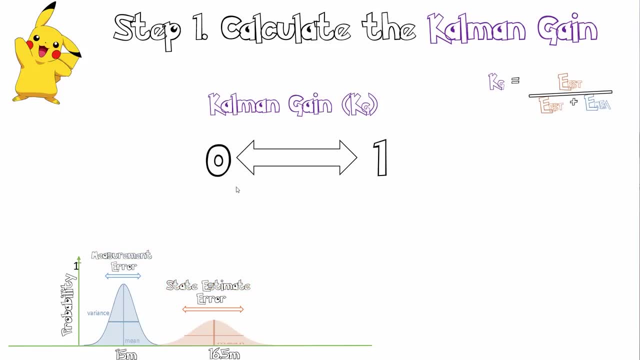 Then our Kalman gain goes to zero. So our Kalman gain is limited to between zero and one where, zero being, the estimate is stable and our measurements are inaccurate, And then we have one where our measurements are accurate and our estimates are unstable. 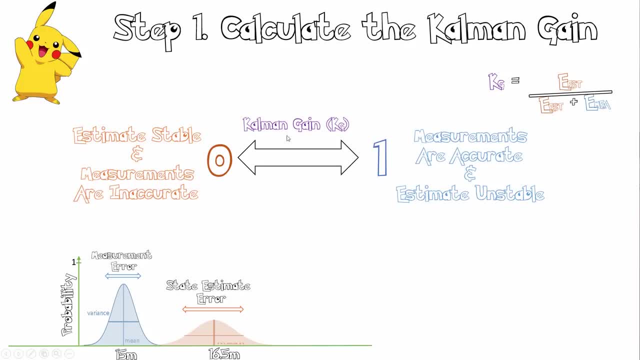 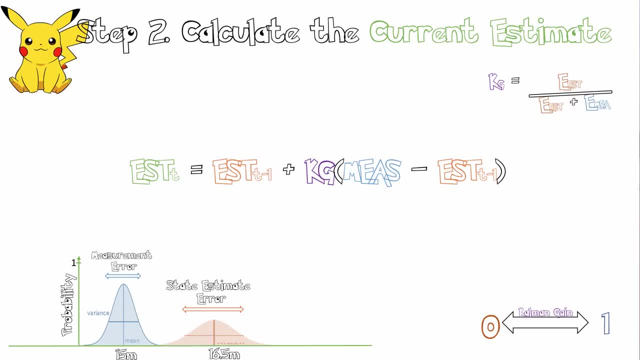 We can go ahead and plug values into this equation and you can see that is true. Then we move on to step two, which is to calculate the current estimate. So over here we have the estimate At time t equals the estimate at time t minus one. the previous position. 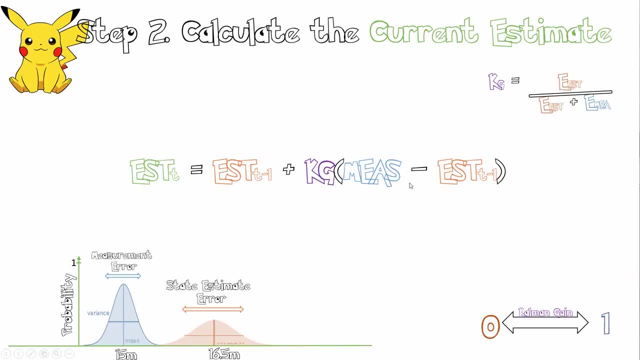 And then we have our Kalman gain, which is the difference between the measured value minus the estimate at t minus one. So that's at the previous time. So what will happen is our estimate will either be between 50 meters or 16.5 meters. between these two points. 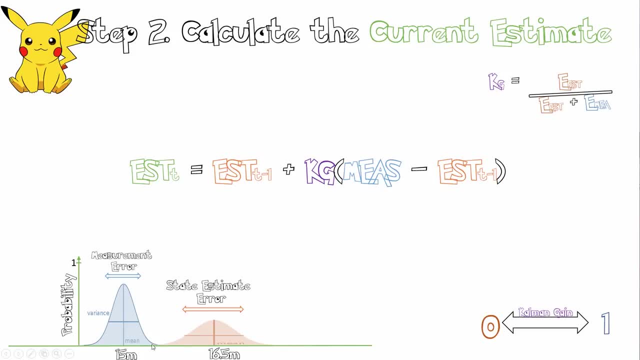 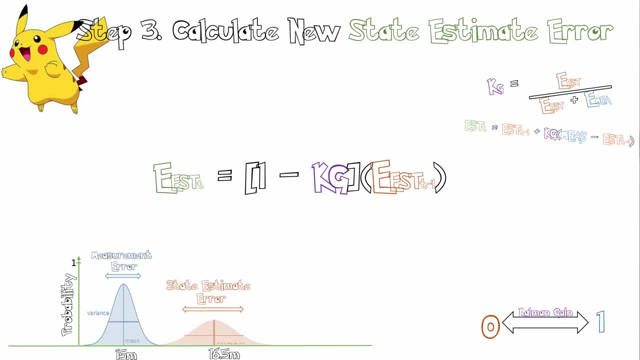 And our Kalman gain will assign a weight that will put it anywhere between these two. And then step three: We want to calculate the current estimate, We want to calculate the new state estimate error. So we have our error estimate at time equals t, which is one minus the Kalman gain. 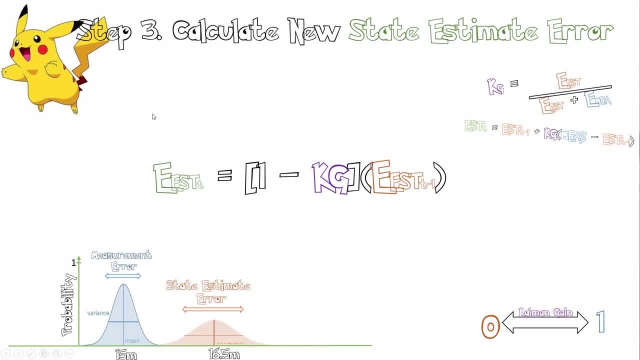 And this is times our error in the estimate at t minus one. So what will happen is the more we use the Kalman filter, the more our error estimate will start to decrease, And that's what we want. We want it to zone in on where the Pikachu will be. 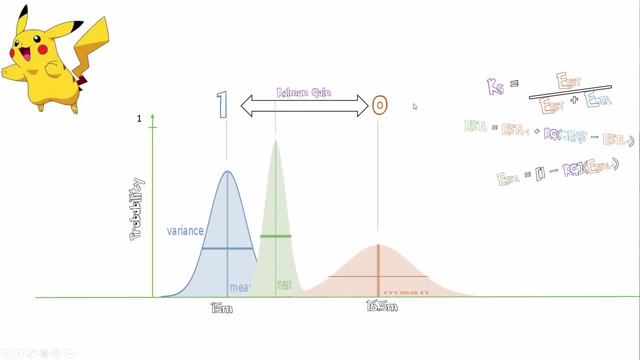 So these are the three basic steps that we need for the Kalman filter. There are obviously much more equations that are involved And how to derive this optimal estimate, But we won't be covering that in this video. But now we're just going to cover the basic concepts. 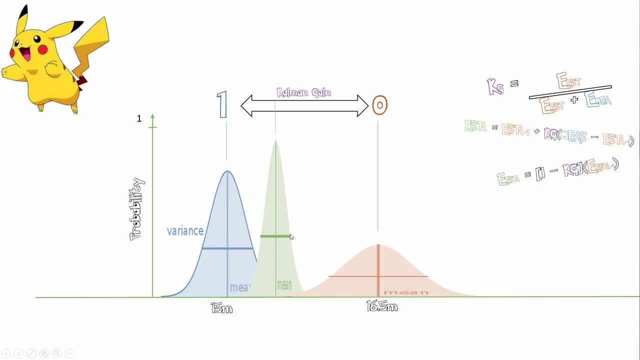 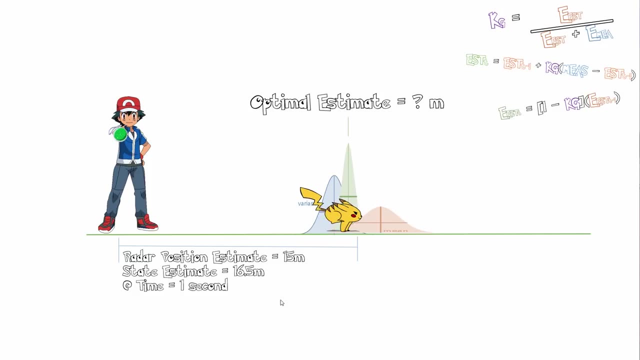 So we've got our measurement estimate, We've got our state estimate And then we've got our optimal estimate. This is what we want to find out Now. using the equations that we just discussed now, we can find our optimal estimate. So let's assume that we get a Kalman gain of around 0.75,, for example. 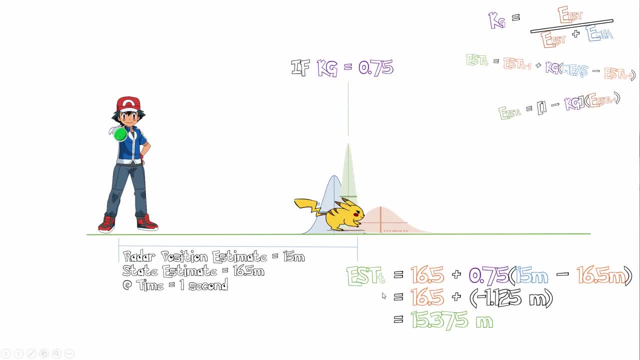 Now we plug that into our equation And what we get is an estimate of 15.5.. And what we get is an estimate of 15.375 meters which, as you can see, is close to our measurement, Since our measurement has a higher probability. 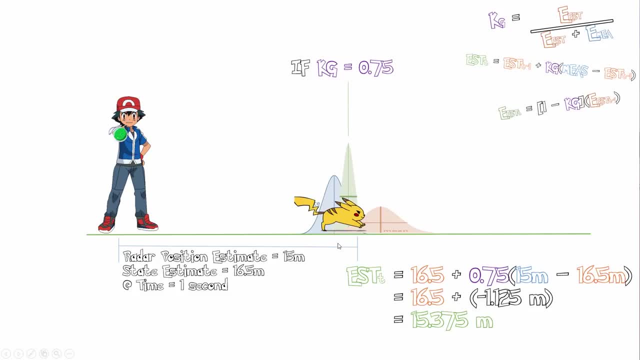 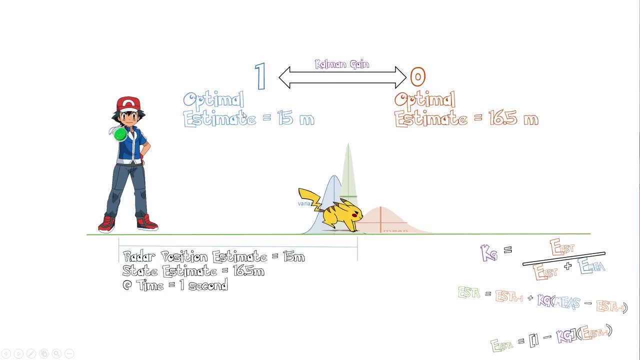 There's a higher chance of our Pikachu being close to the measurement as opposed to our state estimate And, as I mentioned before, depending on what the Kalman gain can be, our optimal estimate can either be at 15 meters or it can be at around 16.5 meters. 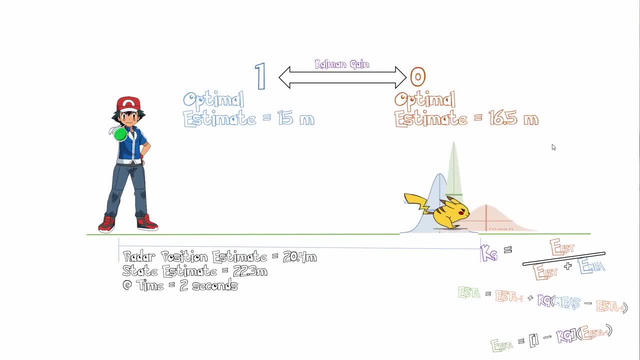 OK, So at time. So at time equals 2.. Let's say, an unfortunate rock Pokemon just drops by And it confuses our results of our Dragon Raider. So now what's going to happen is we're going to pick up the position of the rock Pokemon as opposed to the Pikachu. 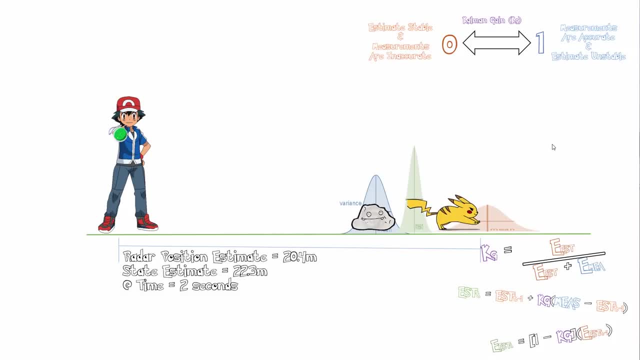 Now what our Kalman filter will do is that it will adjust itself based on what we know about our Pikachu, based on our model. We know that it won't suddenly stop just like that, dead in its tracks. It will carry on with a certain trajectory of motion. 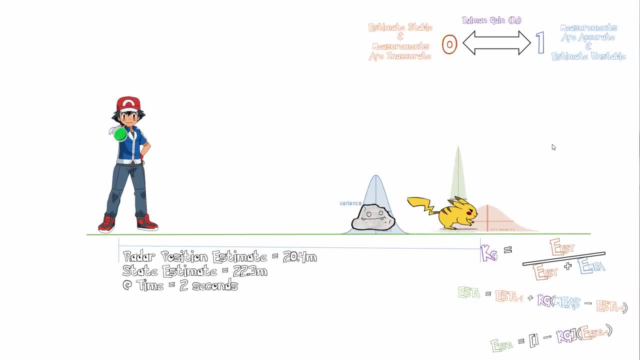 And thus our Kalman filter will move more towards the state estimate. Cool isn't it? And what's really cool about this is that it does this with minimal memory. It means that it just needs the previous state and the current state, as well as the previous error and the current error. 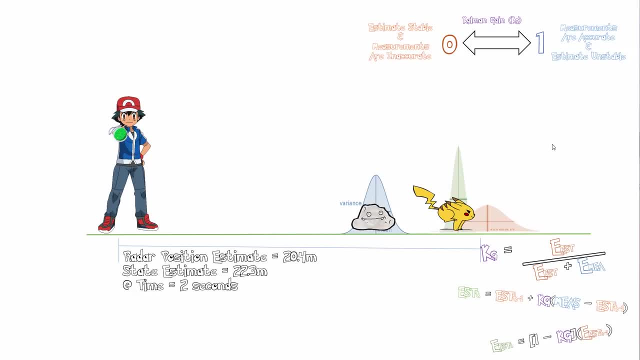 And it can work this out. Obviously there's more mathematics behind how it works, But for now just take my word for it and to why this is so. So again in this scenario. So hopefully after a while our rock Pokemon will leave the scene. 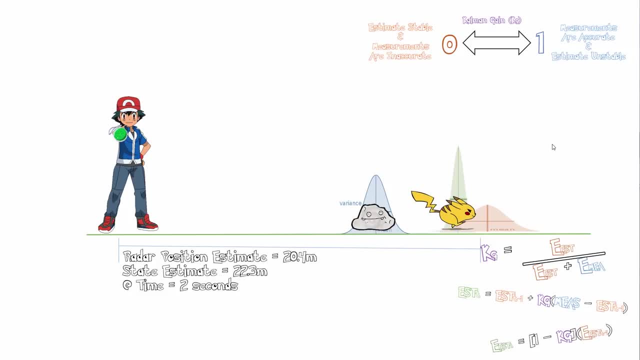 And it won't confuse our dragon raider anymore. This will, in turn, help our Kalman filter to adjust the Kalman gain back to the measurements, Thus providing us with the best estimate of where the Pikachu will be And you can throw the ball knowing safely that you saved a pokeball.